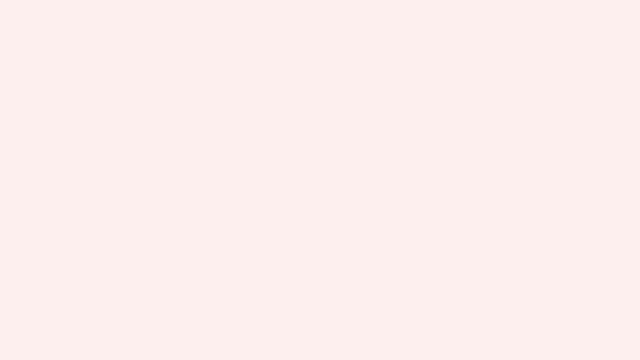 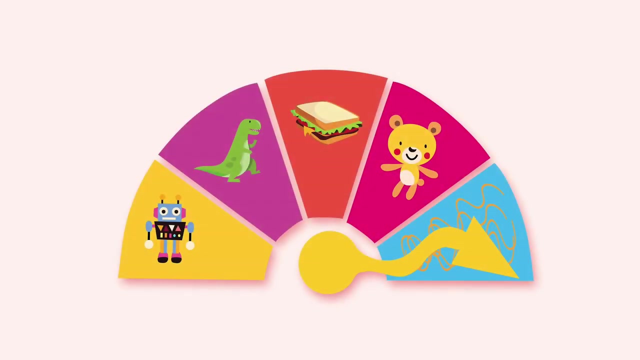 Hello Jamie here. Welcome to Peace Out your place to get real life superpowers that last your whole life. First things first, let's get really comfy. Can you find some space to lie down or sit and spend a moment or so just getting your body feeling totally? 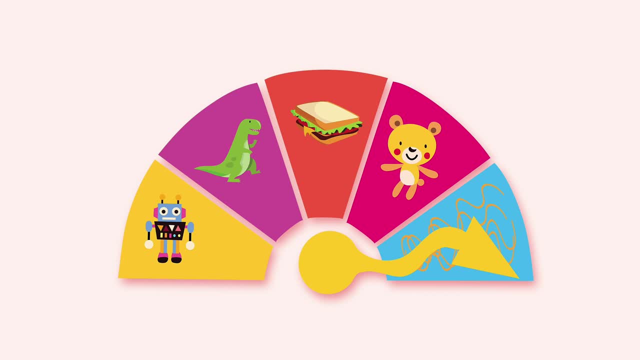 comfortable. Once you get yourself settled and comfy, you're ready to start. So, are you ready? I think you are Okay. then here we go. You're going to find out how floppy you can make your body. To do that, we have a special flop measuring machine called. 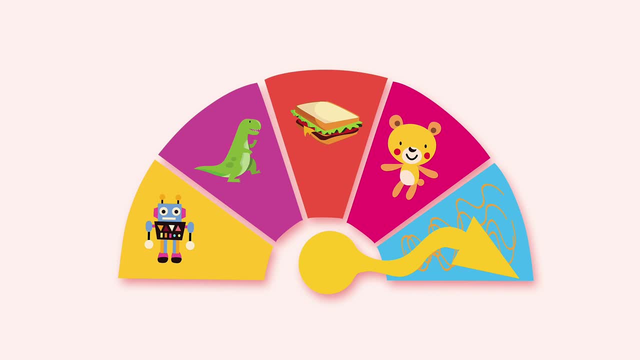 the Flopometer. Can you say that with me? Flop-o-meter. It's a funny sounding word, isn't it? It made me giggle when I first found out about it. The Flopometer has five levels of floppiness, and we're going to see if we. 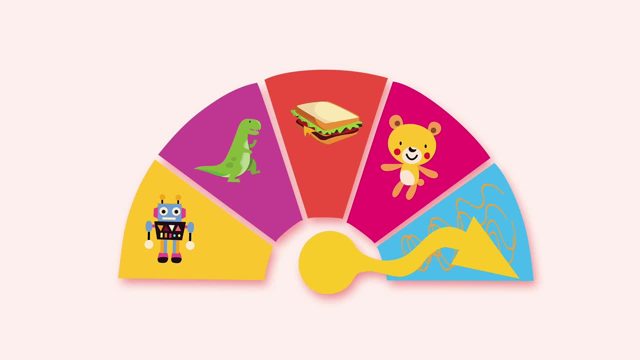 can make it through all five levels today. For every level you do, you get a gold star chime like this: So if you do all five levels, you'll get five gold star chimes, Woo-hoo. Now, if you are super awesome at being floppy and you do make it to level five, let me tell. 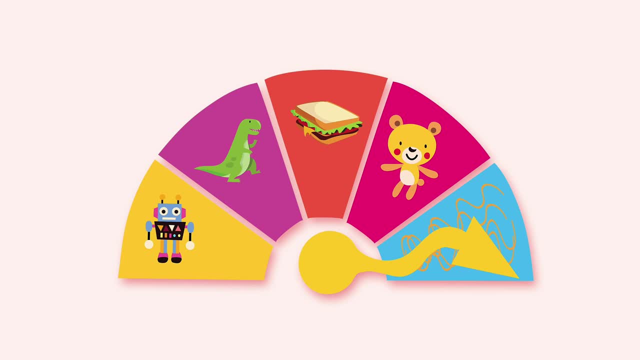 you, you will have reached the top flop spot. What do you think? Are you ready to see if you can do it? I wonder if you'll be able to do all five. Okay, Let's try it out and see. We begin at level one. 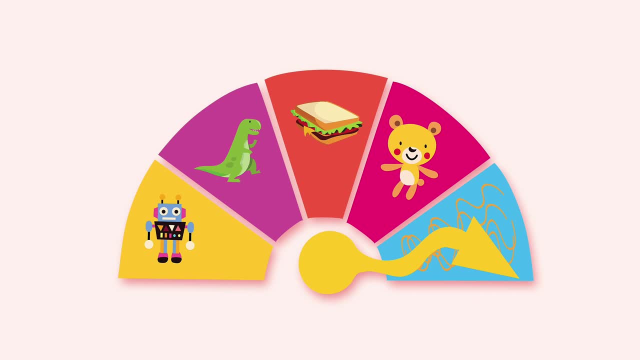 Make yourself as floppy as a robot. Wow, That's not floppy at all, is it? Are you doing it? I'm about as unfloppy as it gets. Everything is super stiff and rigid, Level one complete. Yay, We did it. Well done you. 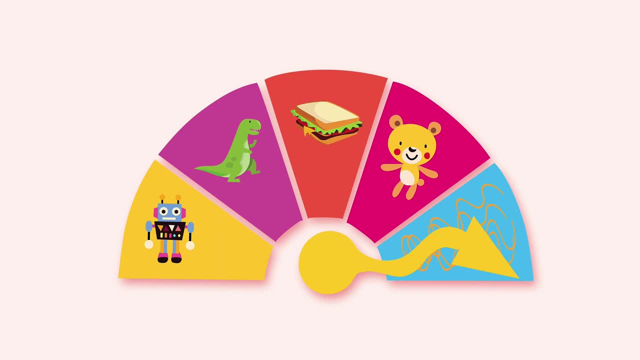 Now let's go for level two. Make yourself as floppy as a dinosaur. Goodness, Still not very floppy. How about you? I feel like I have claws on the ends of my fingers and toes and lots of teeth in my mouth. 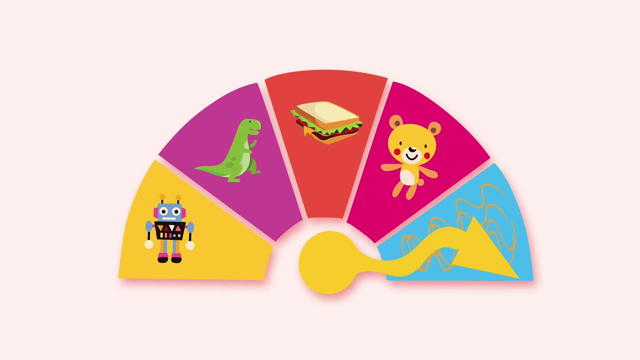 Level two: complete Good work. Next one. Level three: Make yourself as floppy as a sandwich A sandwich. Well, I suppose sandwiches are more floppy than dinosaurs and robots. Let's try it. It feels a lot less tense, don't you think? 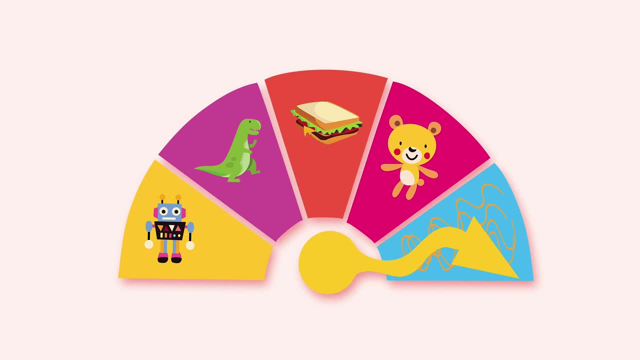 But still a bit stiff so that all the fillings don't fall out of the sandwich. Level three: Level three, complete. Yes, You did it. On to the next one. now, Level four: Make yourself as floppy as a teddy. 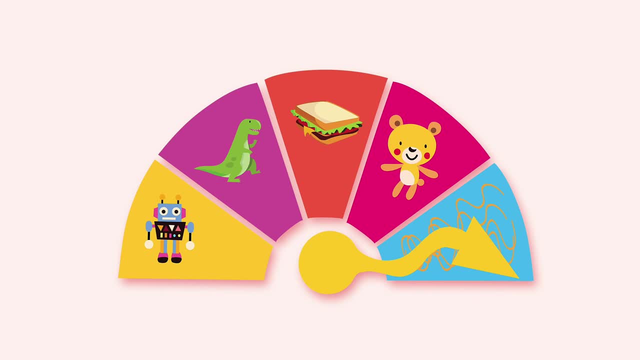 Ah, nice, A teddy. When I think of my teddy, I remember how floppy he is: his arms and his legs and a wobbly head. When I do it with my body, it feels pretty floppy. How about you? 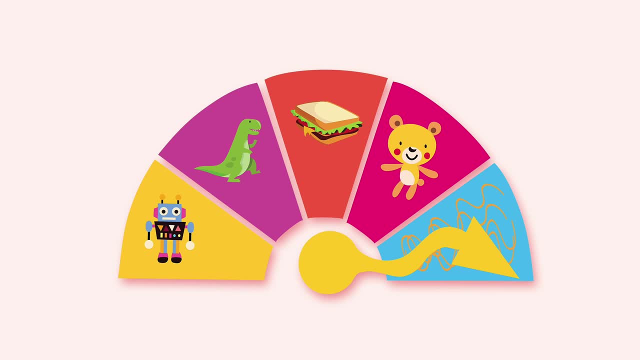 Level four complete. We're nearly there. This is great. We are doing so well on the Flop-O-Meter so far. I wonder if we can be any more floppy. Only one way to find out: Let's go for the big one. 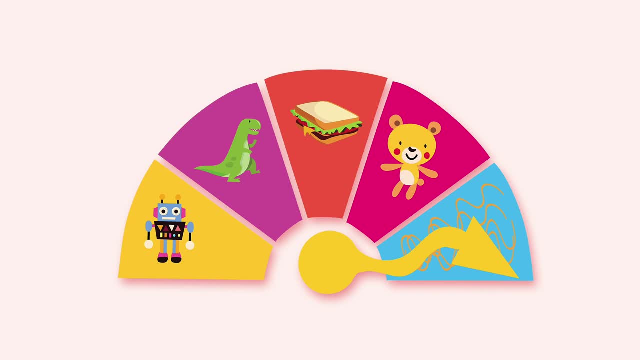 Level five: Make yourself as floppy as cooked spaghetti. Oh, that's really floppy. I'm making my legs and arms as floppy as can be. In fact, I'm making my body really floppy too, and my face. Let's see if we can stay floppy enough to get our final, fifth gold star chime. 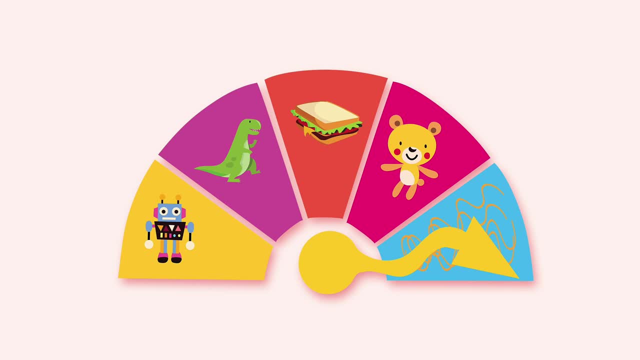 Yay, we did it. We reached level five. Would you like to score some extra bonus flop points? The best cheat for the extra flop points is to close your eyes, Make yourself like the cooked spaghetti again and just breathe slowly In through your nose and out through your mouth. 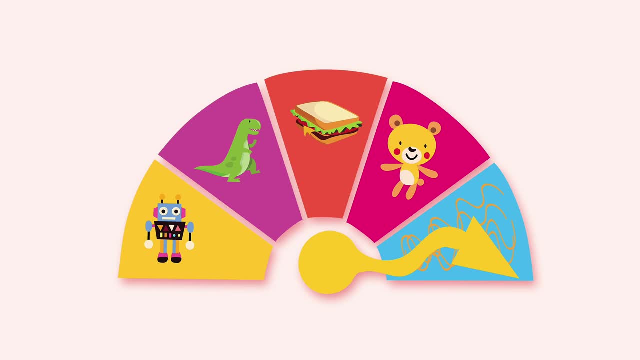 And again in through your nose and out through your mouth. That's it Well done, Wow. did you hear that? That was the Flop-O-Meter telling you that you're the new highest scorer. Fantastic, Now you know about the floppiness levels. 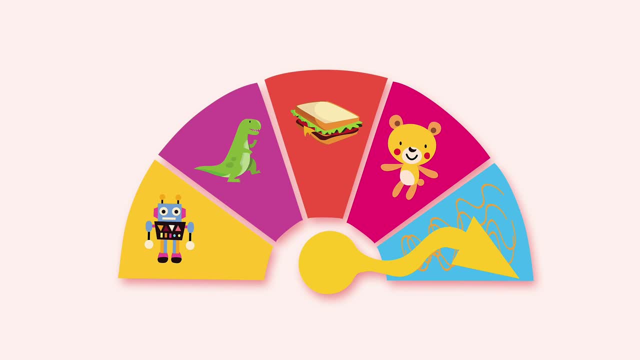 You can help your mind get super ready for our peace outs. Isn't it amazing how your body can affect your mind? But now you know about the special level of flop, You can use it whenever you need. You did so well with the Flop-O-Meter. 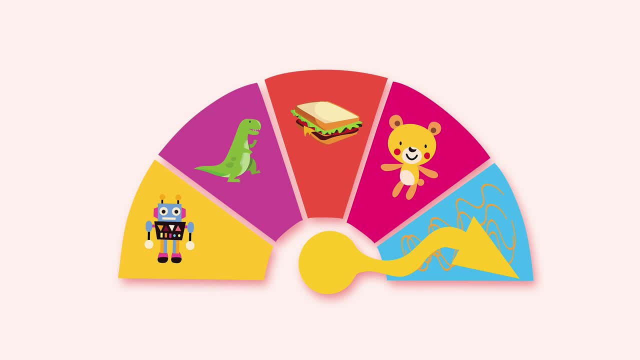 And I hope you found it fun. I did. I hope it helps you too. So the next time you want to think clearly or enjoy peace out, you know exactly how to relax your body, to open your mind. I look forward to our next time. 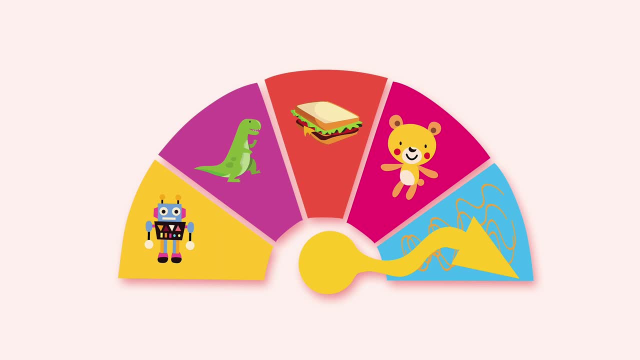 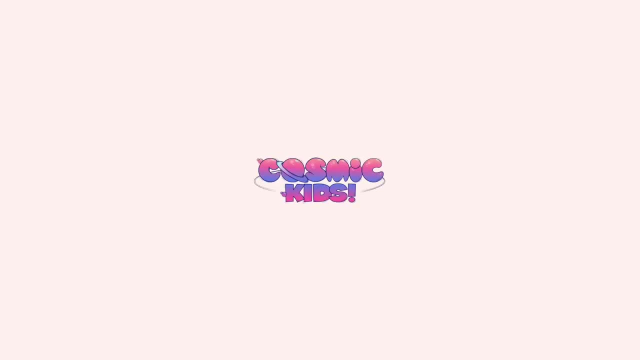 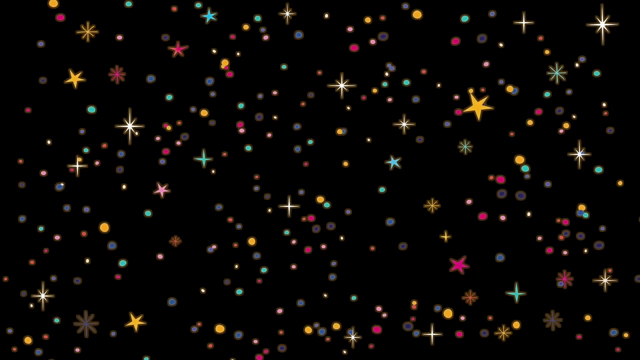 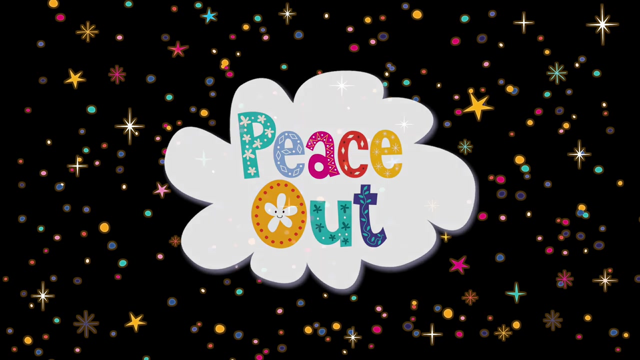 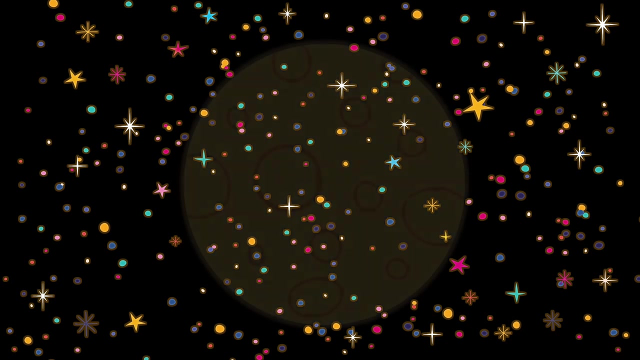 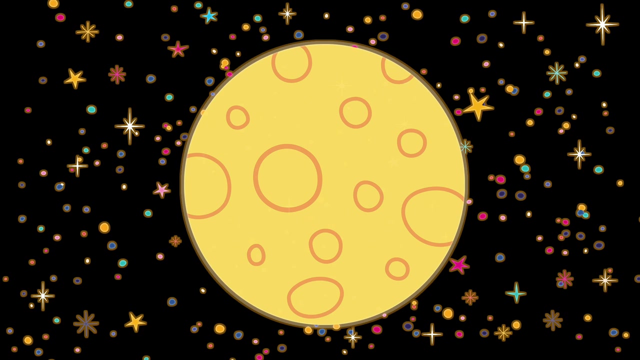 This is Jamie saying: peace out, Peace out, Amen, Bye-bye, Peace out. Hello Jamie here, Welcome to peace out. So which planet' Time to explore the special space in our minds called our imagination? Yes, First, let's get comfy. 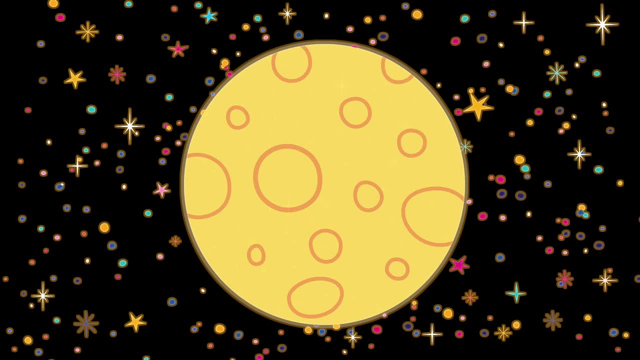 Choose where you want to be Lying down or just sit. You decide what feels good and then get settled. This piece out is pretty good for listening to if you're lying on a bed, So if you can try it lying on a bed. 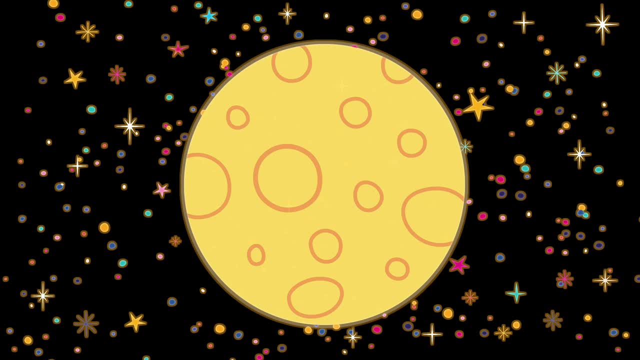 Any last wriggles? OK, have a good wriggle. Go on, Let's get them done, and we'll be much happier. That's it Now. you're really ready. Keep your eyes open and take some big, deep breaths. 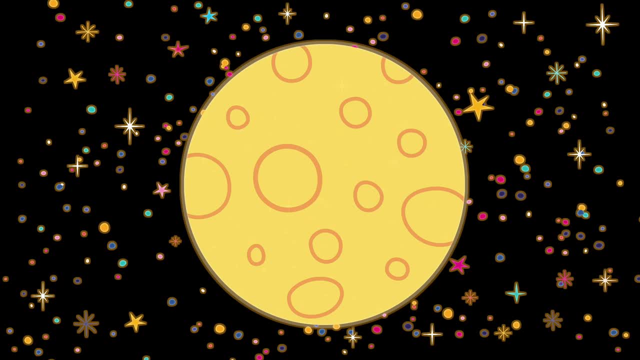 In through your nose and out through your mouth. In through your nose and out through your mouth. That's it. See, if you can take just one more big breath And do this last one as slowly as you can, Breathing in through your nose and out through your mouth. 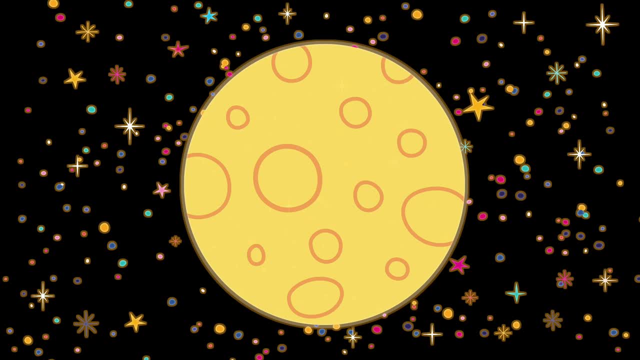 Wow, you really did make it a slow one. That was amazing. The next time you breathe out, let your eyes softly close. Well done, Well done. Let your breathing be normal again And let's see about making our body super relaxed. 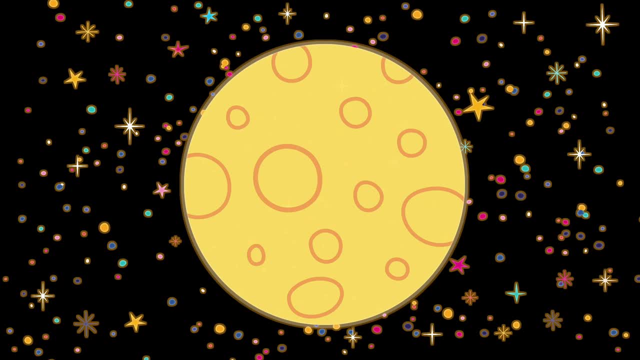 Letting go of any holding or scrunching And becoming as soft as a marshmallow- Really squashy and soft, lovely. Now you're relaxed, You can enjoy letting your mind take you on an amazing adventure. As you listen, the pictures will just appear like you're having a fun dream. 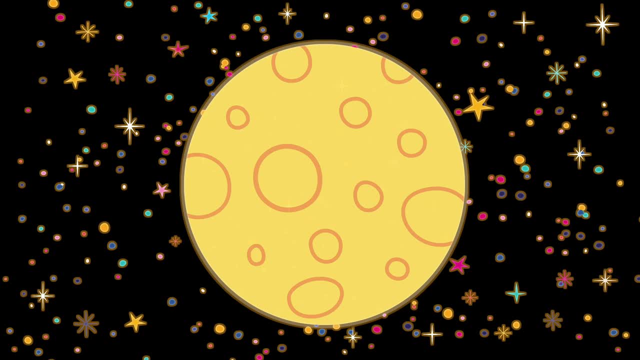 And if you can't see anything in your mind right away, don't worry. Just breathe, Relax even more And keep listening. After a while you'll find it's all happening without you even having to try. Let's go. Imagine you are lying in your bed. 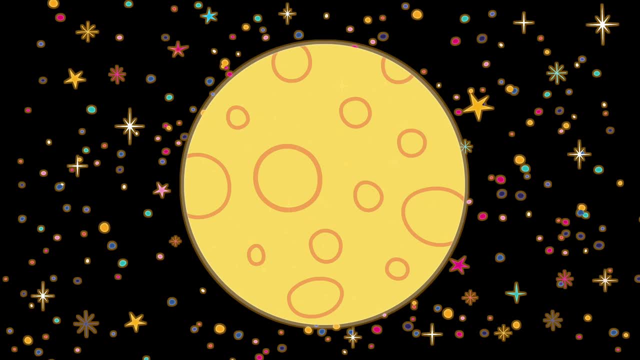 Maybe you really are lying in it, Maybe you are not, Maybe you are. But if you're not see, if you can pretend It's very comfy and warm snuggled beneath the covers. It's night time and everything is so still. 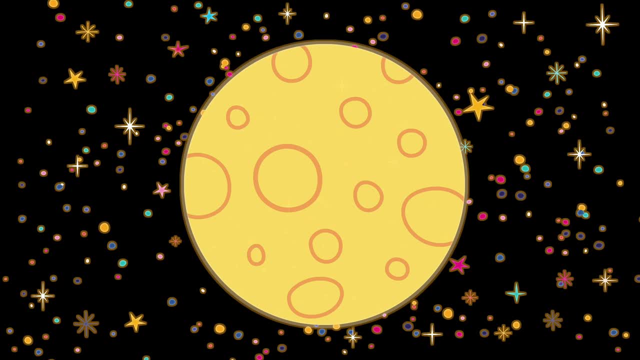 But it's not completely dark. The moon is big and full and bright in the sky And silver moonlight shines into your bedroom through the window- Magic moonbeams down onto your bed. You are looking at the moon. You can see so much on its surface. 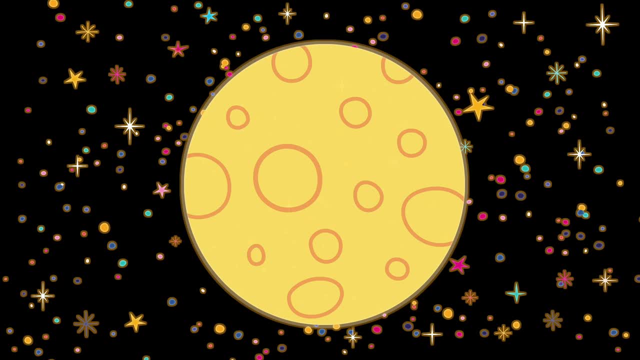 Different shades and patches of white and grey. They must be the craters. you think Doesn't seem so far away right now as you can see it so clearly Now. you notice the stars too, Scattered all around in the night sky. 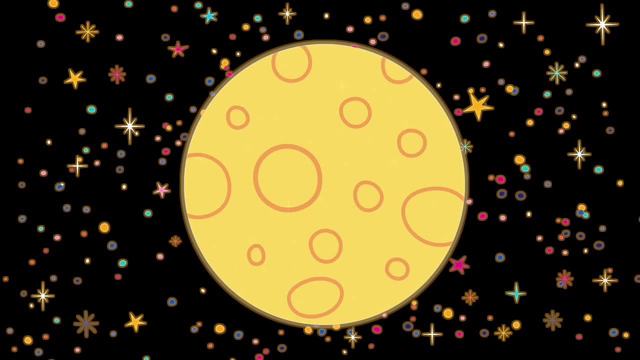 They look like they're twinkling Little sparkly dots jiggling ever so slightly. The more you look, the more stars seem to appear. It's like they are being turned on just for you. The night really is amazing. 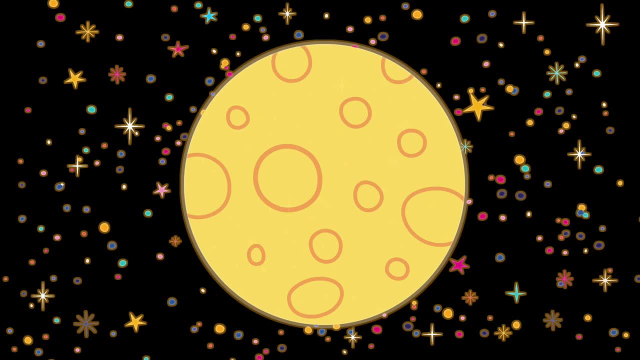 It's amazing. Tonight you see the dark as something you can enjoy rather than be afraid of. There are so many stars now. It feels like they are shining just for you In your mind. you take a big crayon and start to join up the stars. 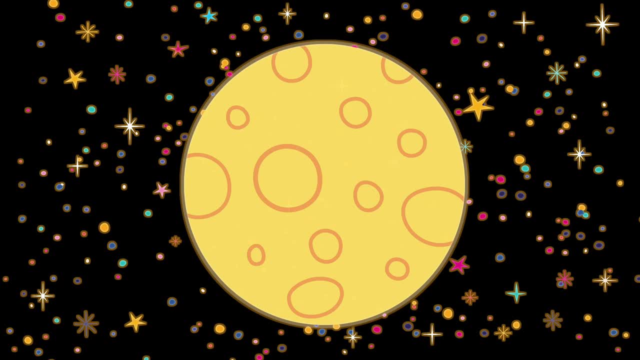 like a giant dot-to-dot puzzle. What shapes do they make? Is it an animal, A unicorn, A house Or something else? maybe Joining the stars together? like this, you are making your own special sparkly star pictures. The night sky feels like it belongs somewhere. 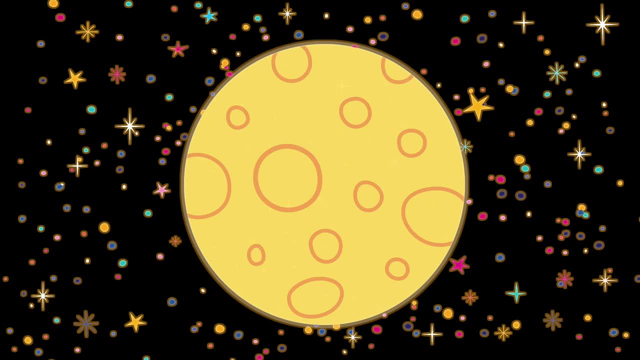 A mirage gets attached to you and the moon beams brightly smiling down at you. You feel so very tired now And ready to drift off for a good rest. The beautiful starry night sky above you will always be here, even when you can't swim. 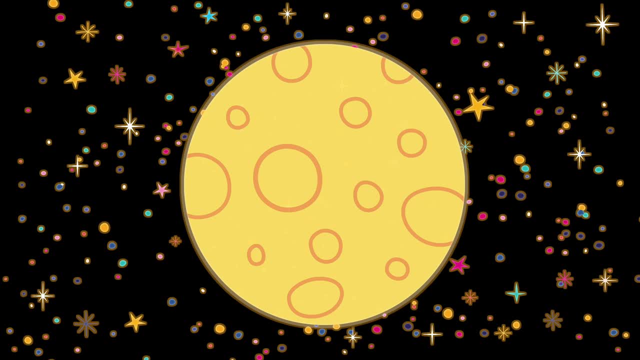 And on the other side there is the old moon. see it, for the clouds, Know that. the sparkling stars are always there, and the moon too, beaming down, sometimes full and round, other times only half full or just a little curve like.